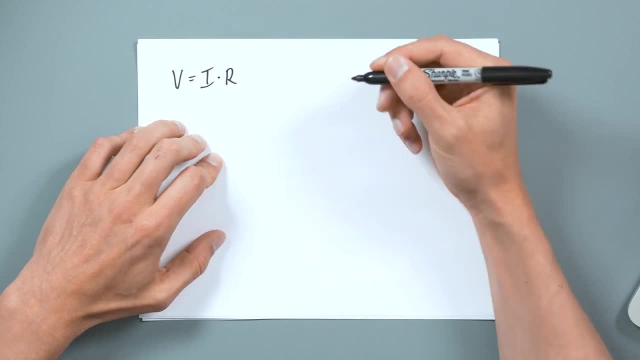 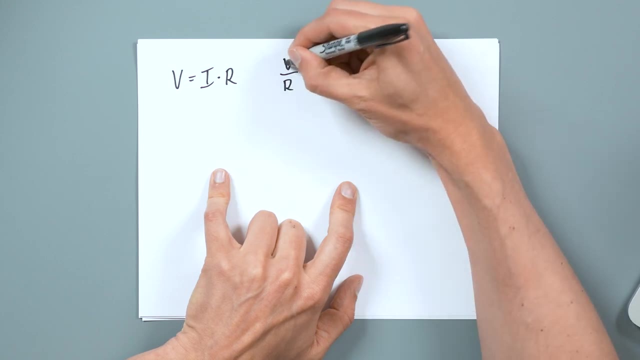 the current I times resistance And that can very easily mathematically be switched. So you have voltage over the resistance. that V looks terrible, as always- equals current And you know honestly we could do. voltage over current equals resistance, You can move. 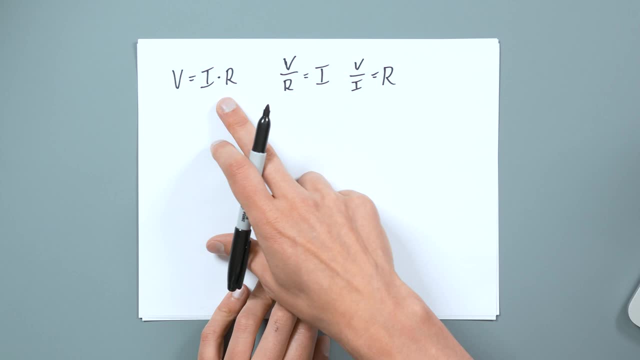 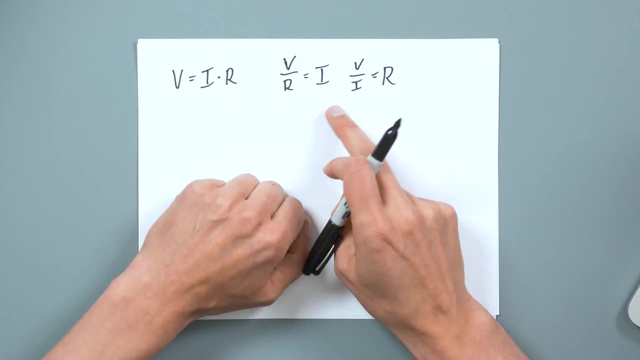 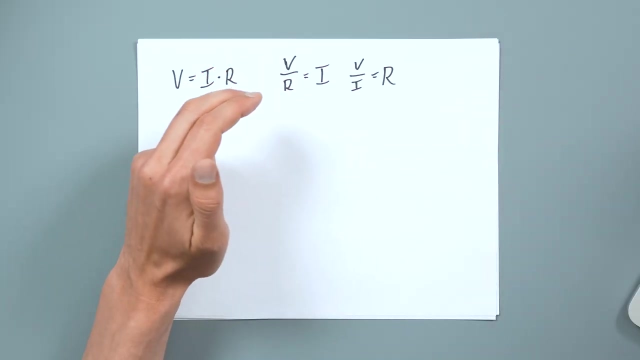 this thing around however you want, but I typically like to see it in this way. It's a pretty way for me, but, honestly, the voltage over resistance equals current. It's probably the best intuitive way to understand this And, as you can see here, so if you have a voltage and you lift that glass higher, if 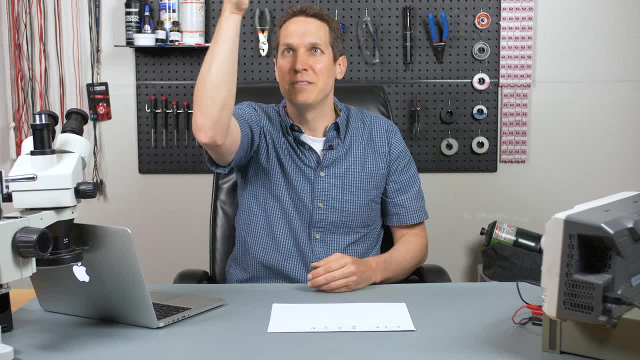 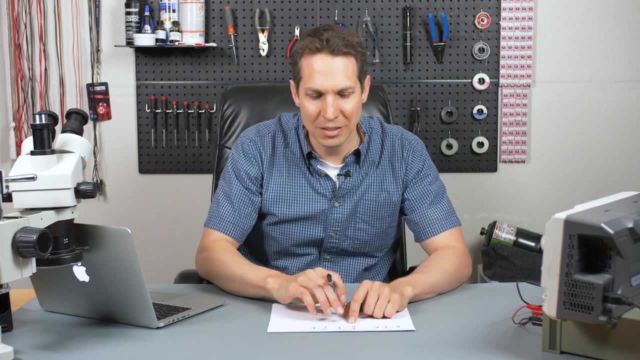 you have the same amount of resistance, you're going to have more current. But if you have a voltage and you increase the resistance, you're going to decrease the current. So one of the things about this is: you'll notice this is a very linear relationship. If you 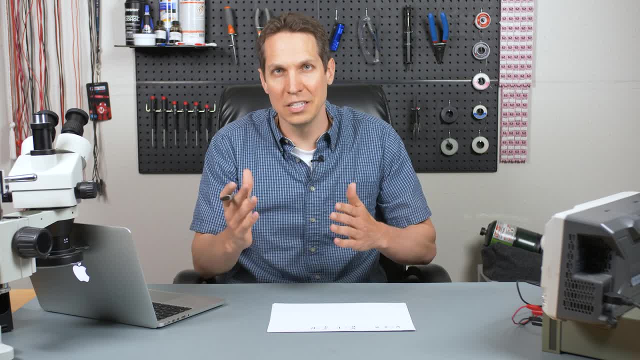 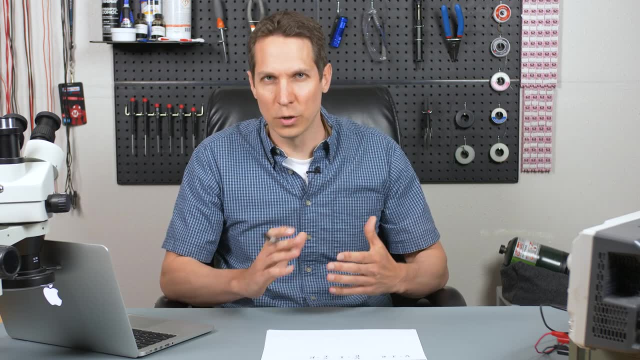 change any of these. the other things are going to change linearly, And this is not the case with a lot of components. but with resistors we typically treat them as linear and we don't really worry about those other cases in the vast majority of time. So voltage: 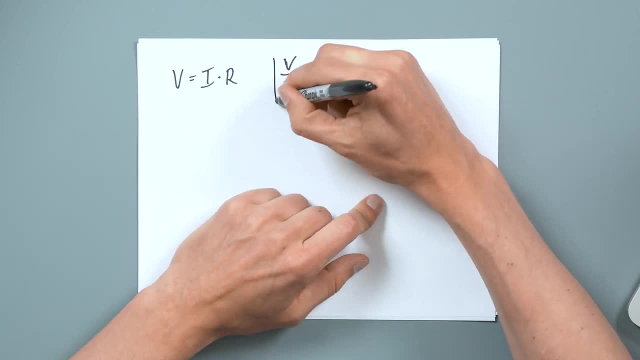 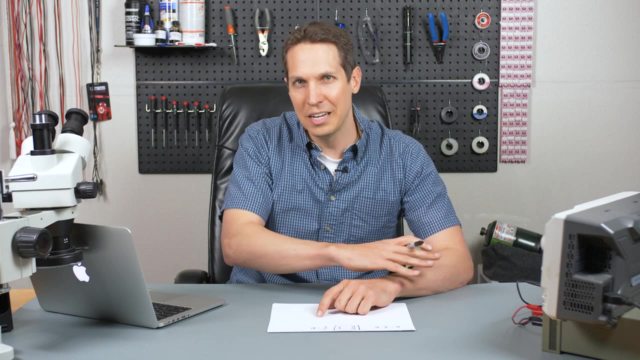 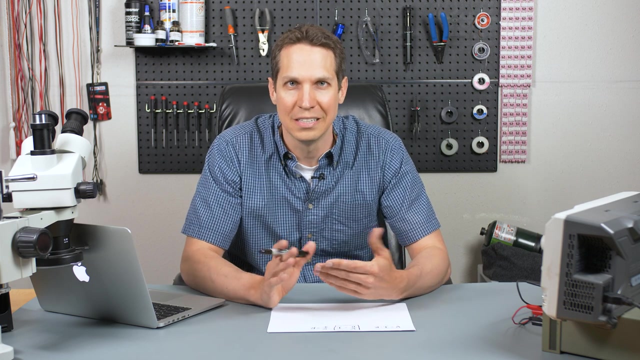 over resistance equals current. This is so huge It's going to be used in basically everything- every circus class from here until forever, And then a lot of the things in electrical engineering still refer to this, even if it's not circus related. So this is an incredibly important thing and also very straightforward. 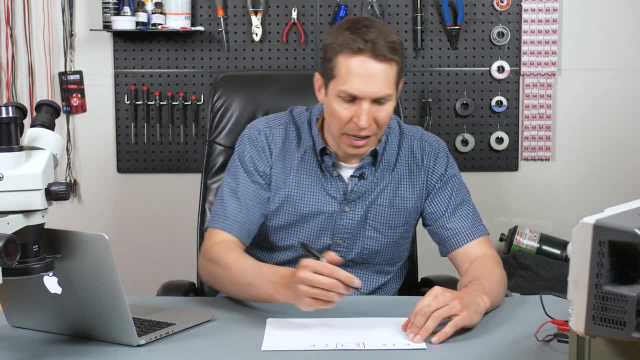 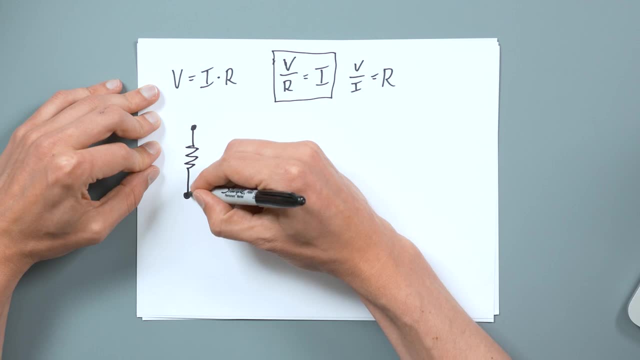 and you're going to learn a lot about it. but let's go over it a little bit more. So if you are given a circuit, let's just put a node right here, a resistor and then another node. we already have everything we need to solve something. 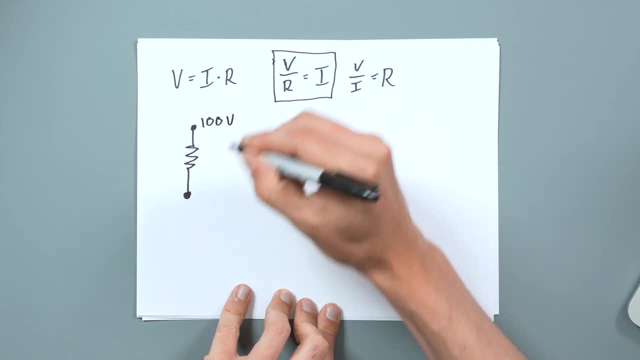 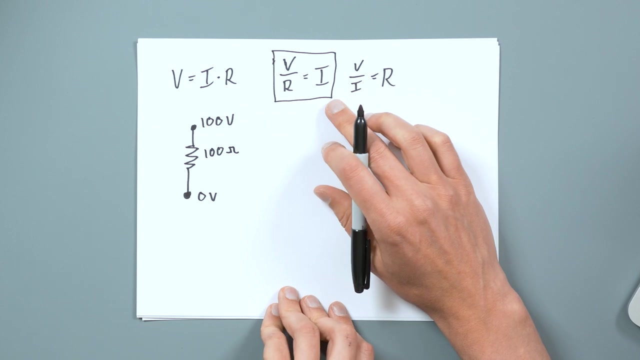 So let's say this is going to be 100 volts and this is zero volts. So now we have 100 volts across this resistor. And then let's say this resistor is one hundred Ohms. We can use Ohm's law to very easily say: okay, we have the voltage and we have the resistance, So we'll want. 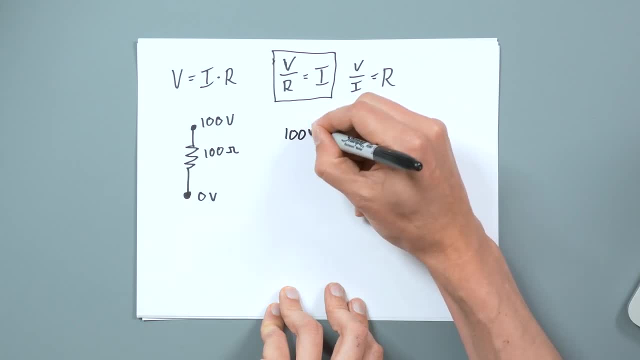 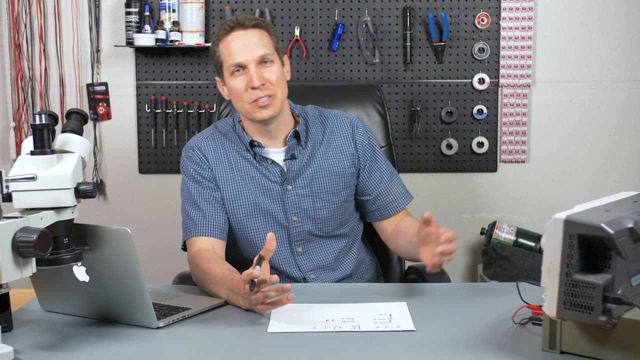 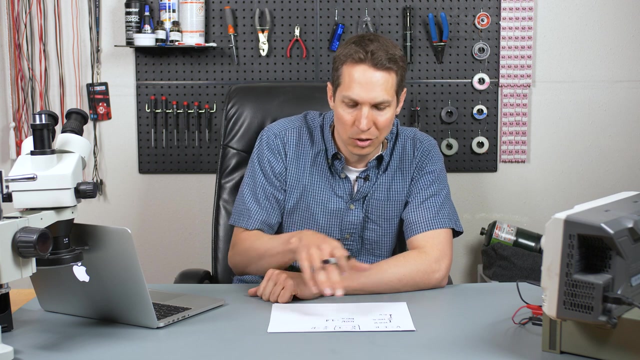 to use this format, We'll say 100 volts over 100 Ohms equals one Amp. Okay, That seems super simple And it is super simple. It gets much more complicated, but that is the essence of how you can use Ohm's law to solve for the current Or if. 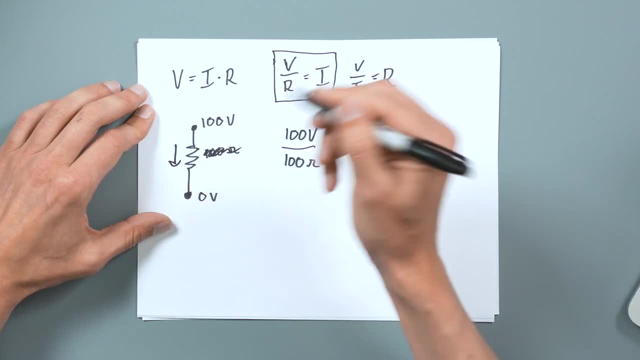 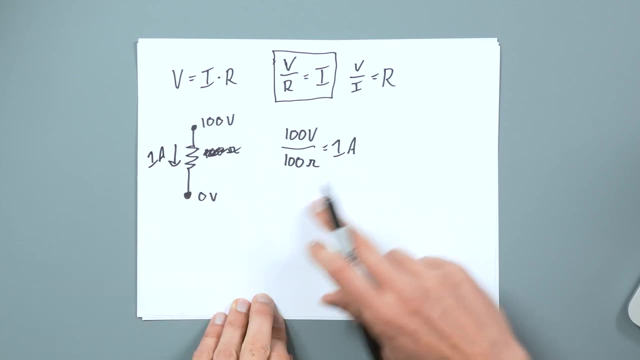 you happen to know, if you happen to know what the current is, then you can do the same thing of saying: oh, I know I have one amp through here and there's a hundred volts across it, So whatever I need, so you can use any of these, you just need to have two, and then. you'll figure out the other one. So this is pretty simple. I'm going to go ahead and do that. I'm going to go ahead and do that. I'm going to go ahead and do that. I'm going to do that. I'm going to go ahead and do that. I'm going to go ahead and do that. I'm going to do that. 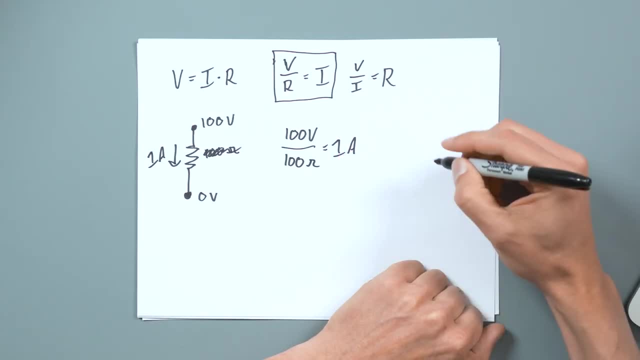 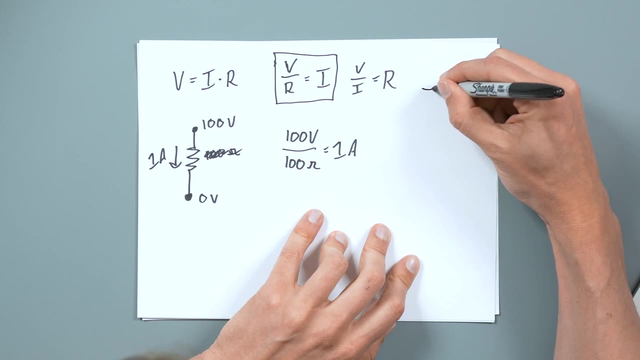 So this is pretty simple And you notice I use the word Ohms and it's wow. That is, and I apologize, My handwriting is so, so bad, but this is a Greek Omega. Let's see if it can look a little bit better. No, that just looks like some sort of farming implement. 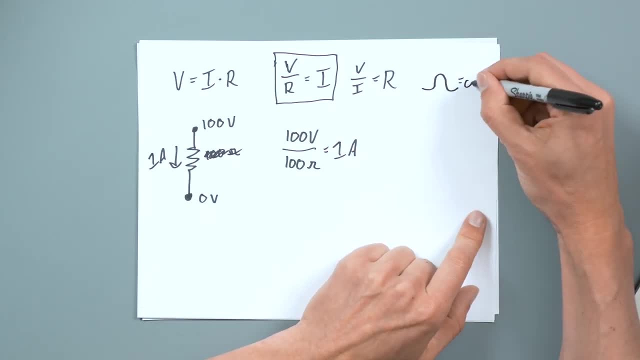 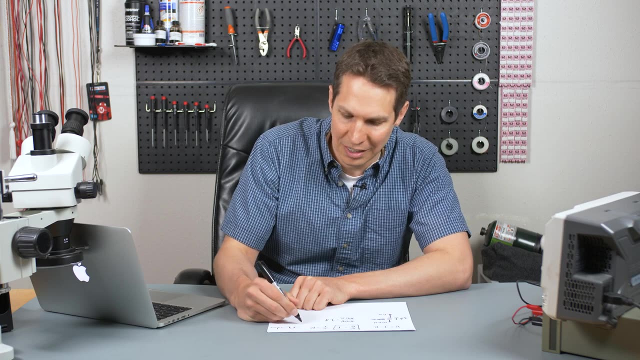 now. But that is what that symbol is. That means Ohms, and that is the measurement of resistance. Now there's actually something out there that is called a Mo, and it's an upside down. Oh my goodness, That's really going to stretch my ability. 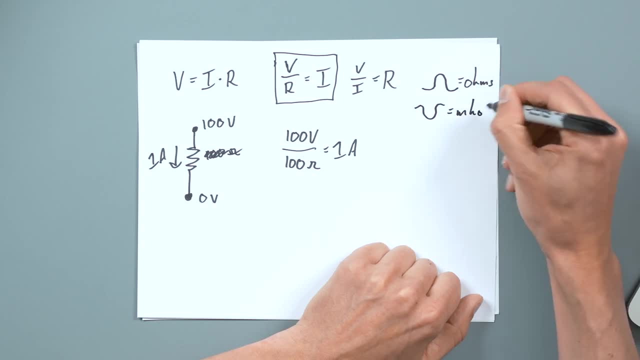 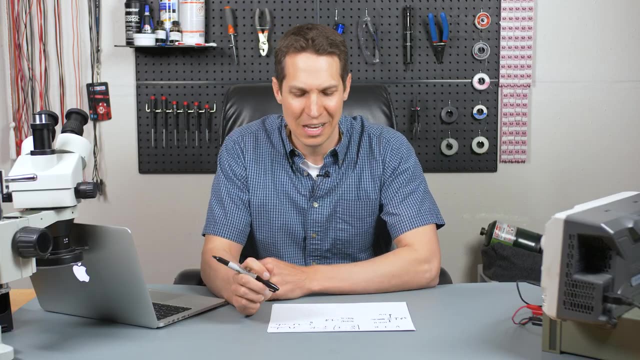 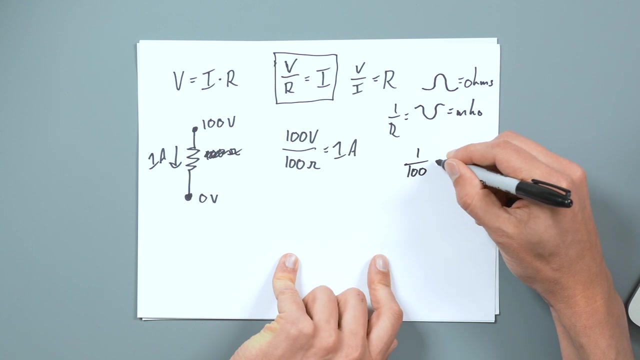 And that is one over R and that is called conductivity and that can be Mo's or Siemens, whatever you want. So 100 Ohms would be one over 100 Siemens, And that's just an S. or you can also do one over 100 Mo's And you're not really going to see that that often- At least I haven't, If you. 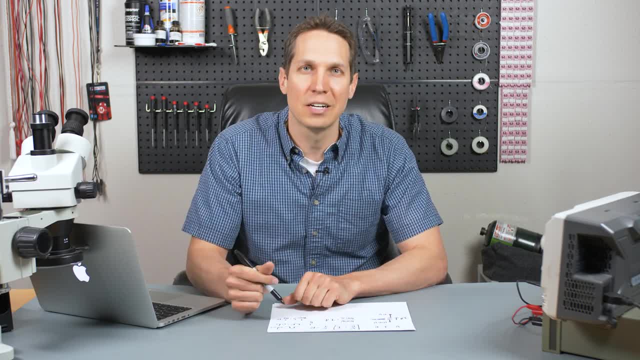 do. you'll see that. So that's a good thing, And that's what I'm going to do, And that's what I'm Well great, I'm glad that I've introduced it. But you might hear that on occasion. 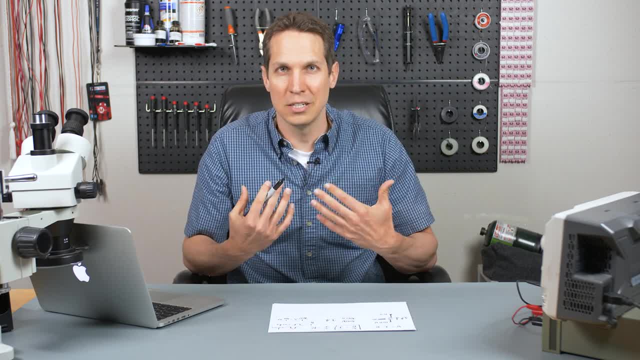 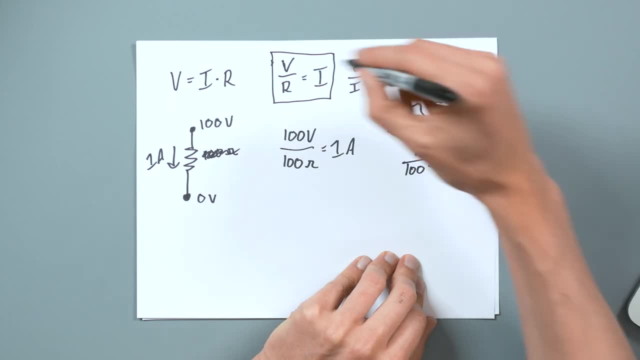 That's the only reason I wanted to introduce it to you. But in my career and in my time in college I very, very rarely saw that. So if you do that, you can totally change Ohm's law to again follow those rules. 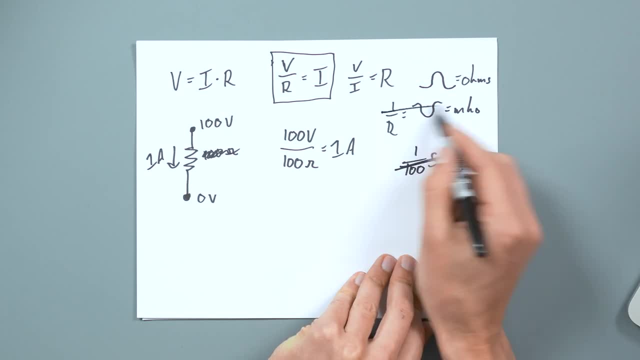 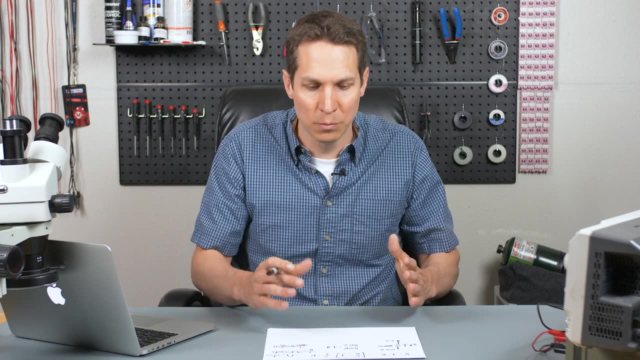 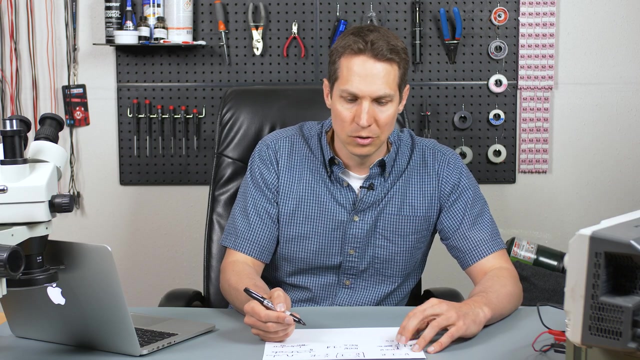 But now that I put that out there, we are going to completely ignore this ever again. So enjoy. So before we get into the samples, I just want to give two cases of the extremes of Ohm's law. So if you have V equals IR, imagine your R is zero. 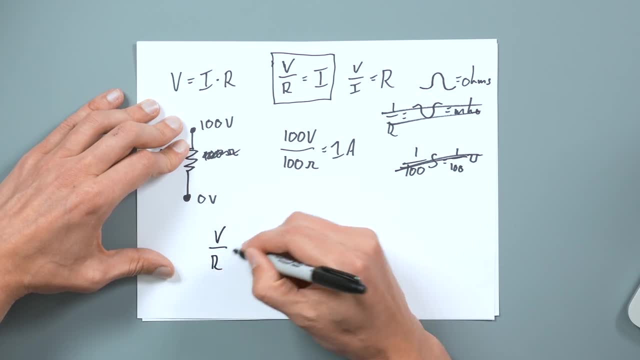 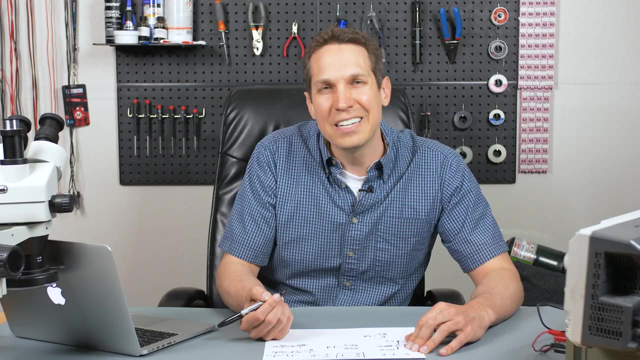 So you have V over R, which equals zero. what does that come out to be? comes out to be infinity, And that is called a short circuit, And that's something what happens if you take a battery and you just put a wire from one. 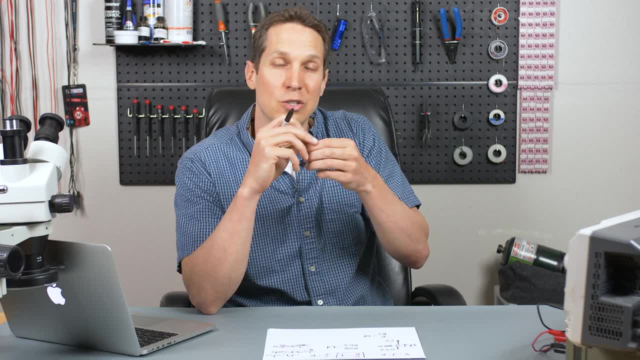 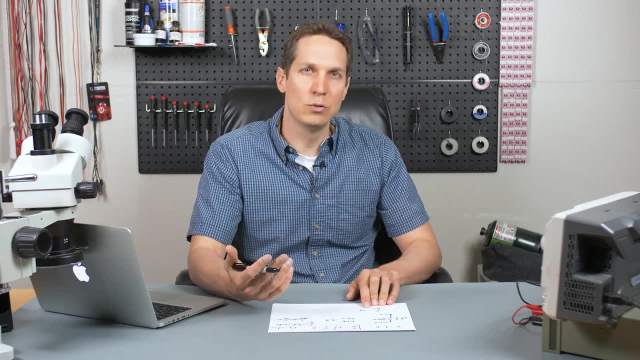 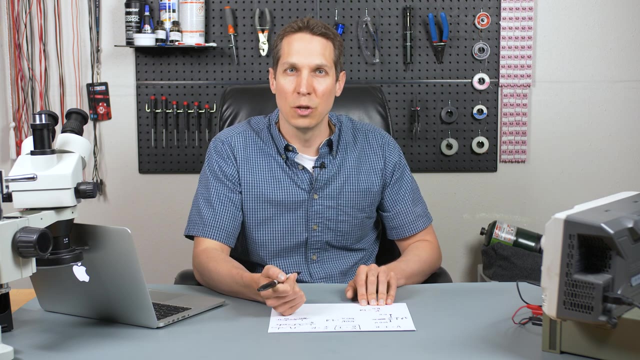 end to the other. that wire is essentially zero resistance, So that battery outputs as much current as it possibly can until it melts and everything goes away. In most cases you don't want that. Some cases you might. I think when you are doing welding they try and get that- is that resistance as low as 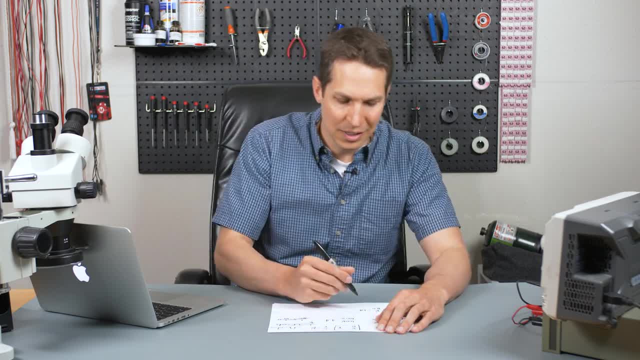 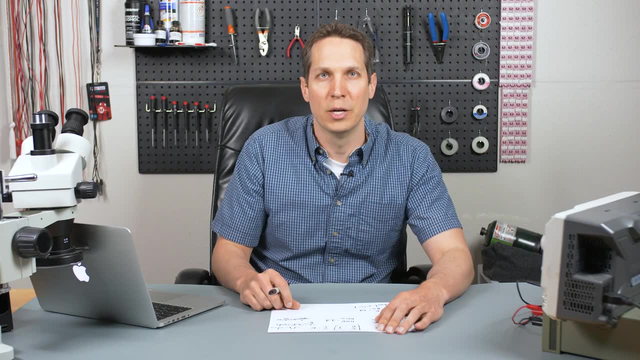 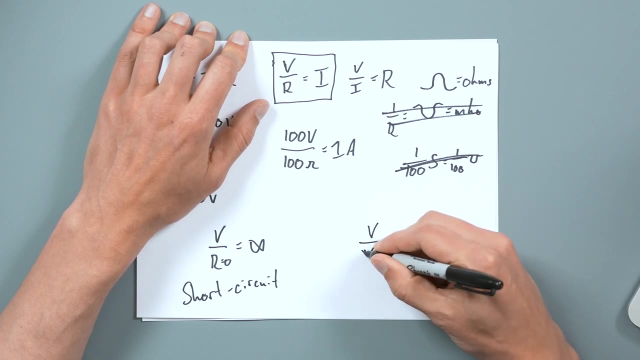 possible so that they can get as much heat there as possible. But this, in general, is something we want to avoid, because it usually means your circuits about to blow up. Now let's say we have the opposite problem: voltage over infinite resistance. Okay, Okay. 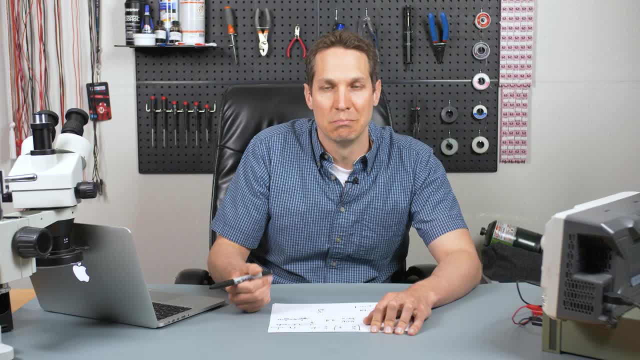 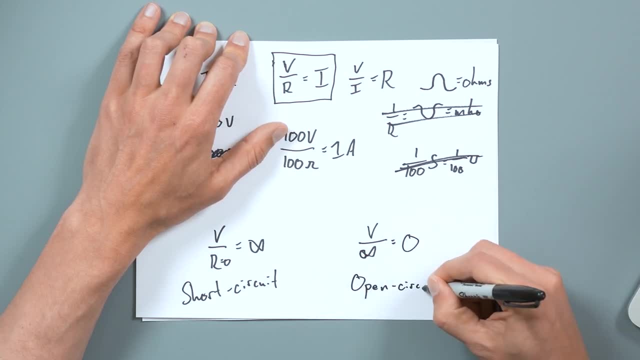 There we go. Then what is our current going to be? It's going to be zero. Get the exact opposite, And this is called an open circuit. Sometimes this is what you want, Sometimes this isn't what you want. Sometimes, when you have a circuit and you're testing things and you are not getting any, 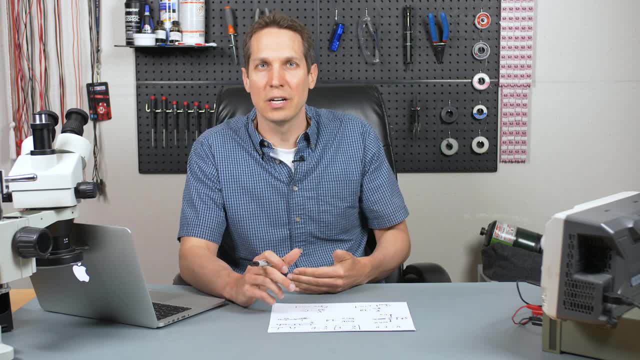 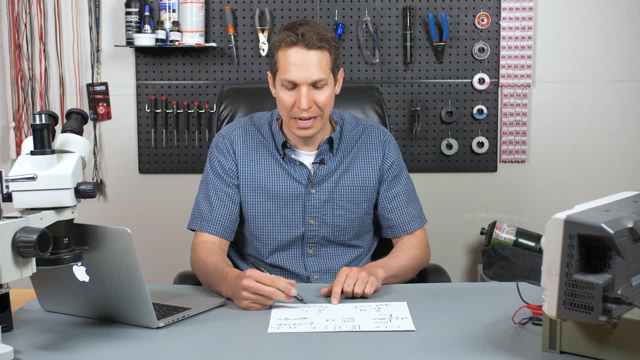 current, it's like: oh okay, that means that I have an open somewhere in this. And if it's on your circuit board and you can't see where it's broken, that's a problem. But at least you know from there being a complete lack of current that is an open circuit. 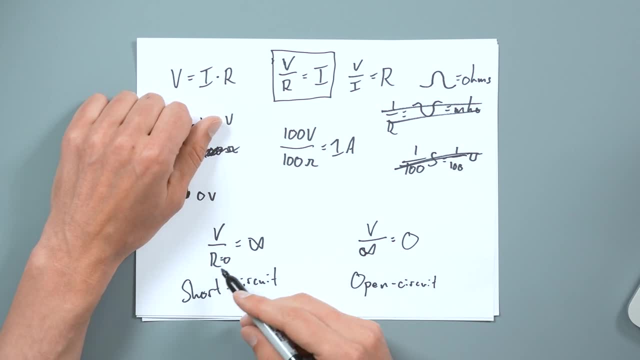 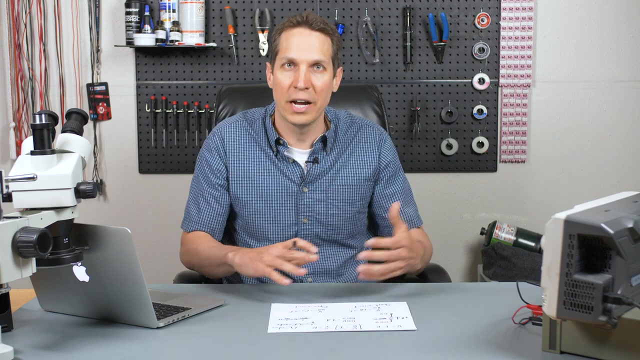 These are the two extreme cases of Ohm's law- when resistance is zero and when resistance is infinity- and how that affects your current I. So, with that out of the way, let's actually jump into a couple of examples so we can see how this is used practically. 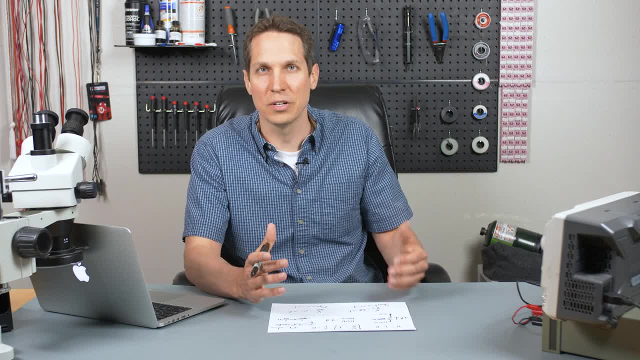 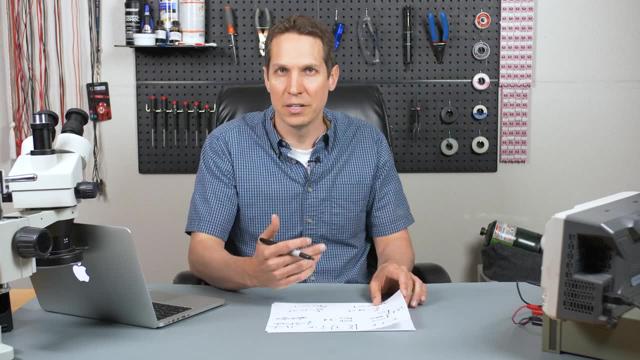 Now we're not going to be able to solve anything crazy or anything truly that interesting until we learn a couple of more tricks, but at least we'll have a couple of examples of how to do Ohm's law in very simple circuits. Okay. 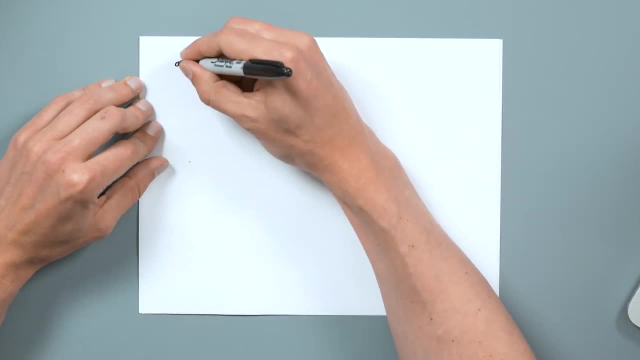 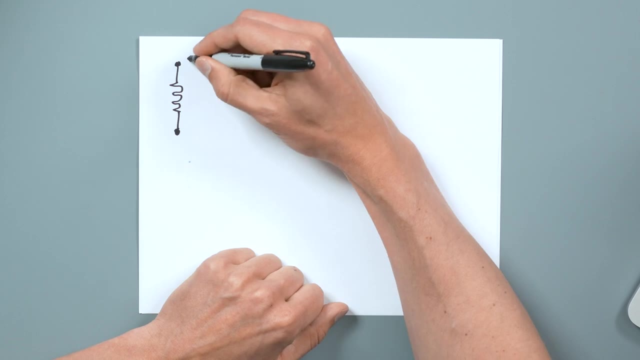 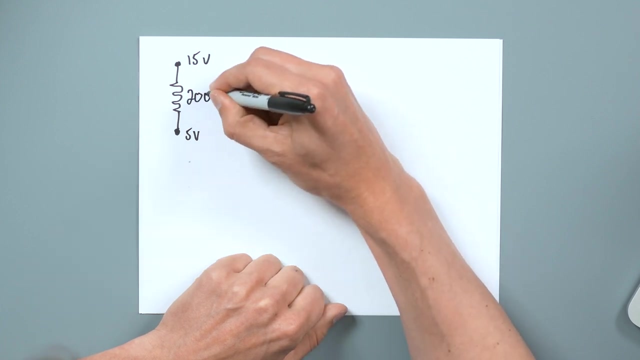 So the first circuit that I'm going to set up here is after that super simple circuit that we had. Oh man, Okay, I'm just going to stop complaining about that and keep on going. We are going to have 15 volts here, five volts here and 200 Ohms right there. 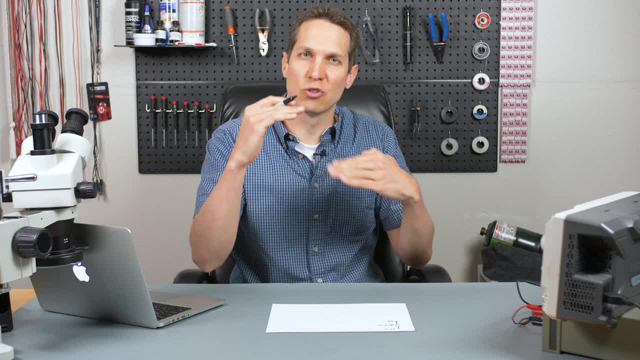 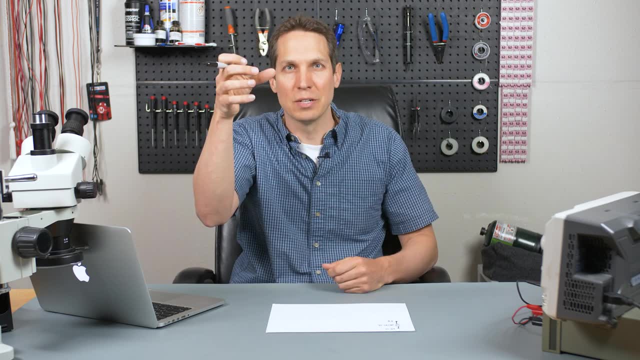 So when you're dealing with voltage potential and it's that voltage across something and that's what's important. So when I'm holding the glass here, it doesn't matter. I'm actually in the basement right now because all I care about is from here to here. 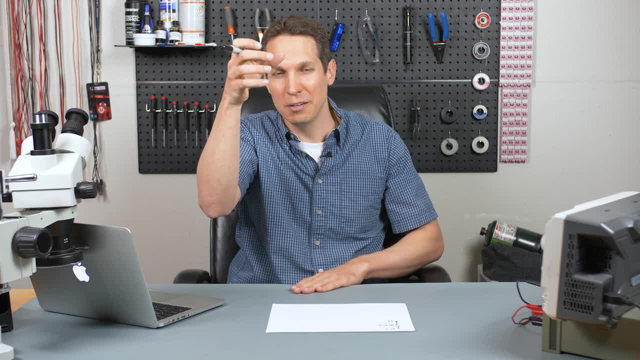 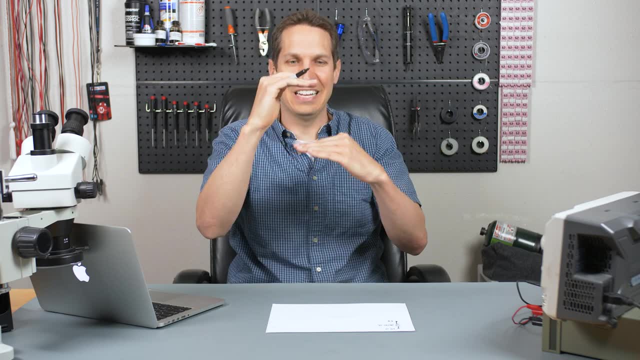 Now from here to here, was sitting on the roof of my house or on the roof of our office, That distance is still the same. So voltage potential can move like this, And as long as that distance between the two points is the same, it really doesn't matter. 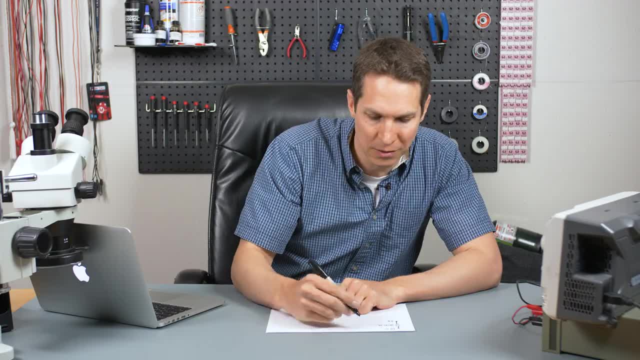 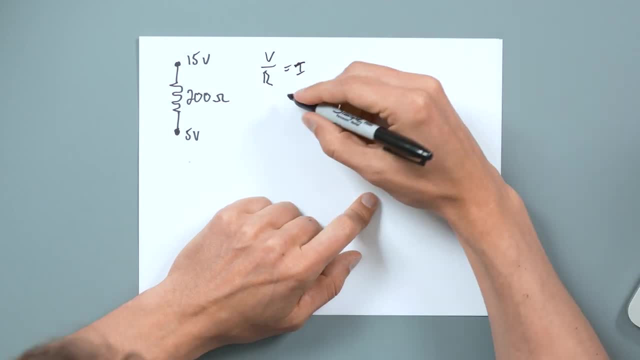 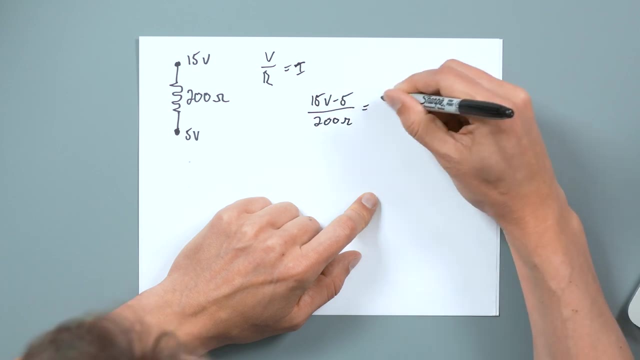 So, with that in mind, let's look at this. and now we are going to have: our V over R equals I- Whoa, that's a one. But now our V is actually 15 volts minus five volts over 200 Ohms, which equals 10 volts. 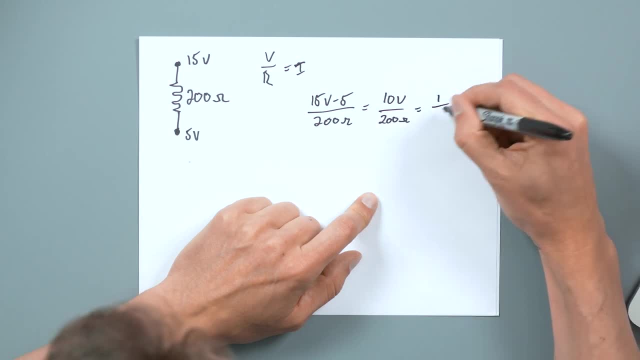 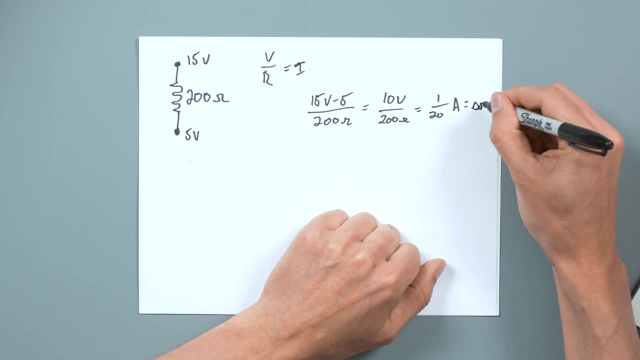 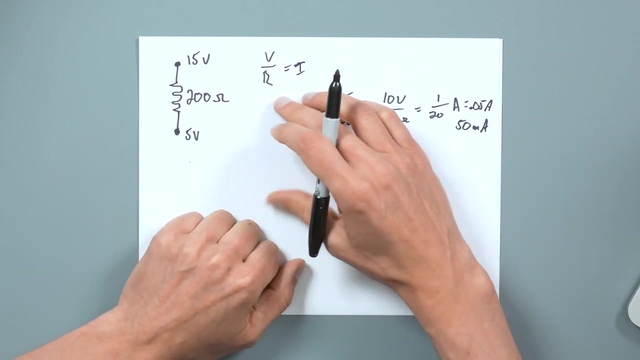 over 200 Ohms. So now we're just getting 1, 20th, 1 over 20, which is about 0.05 amps or 50 milliamps. So the key thing that I want to take away from this is: it doesn't matter that this was. 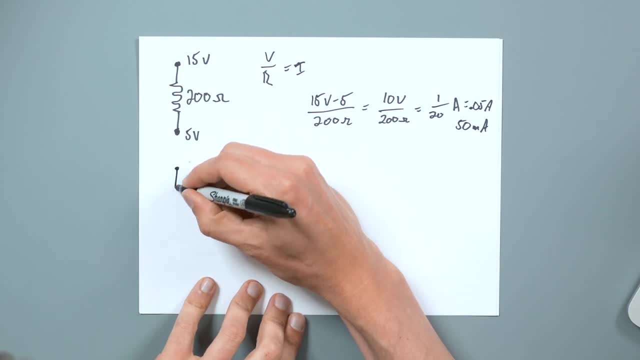 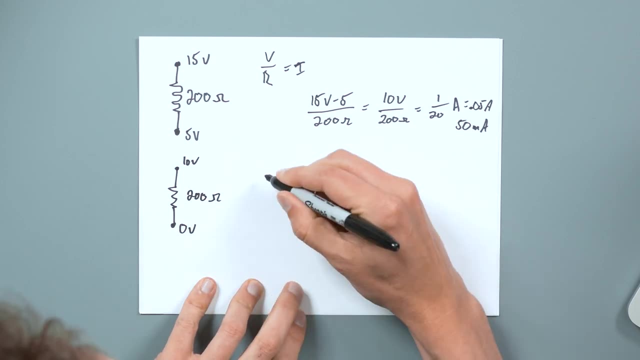 15 volts. It doesn't matter that this was 0.05 or 5 volts, because we could do this exact same circuit at 10 volts, 0 volts, 200 Ohms, and then we'd still have 10 volts minus zero over. 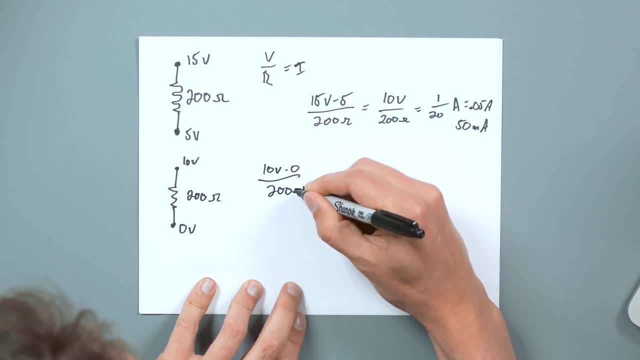 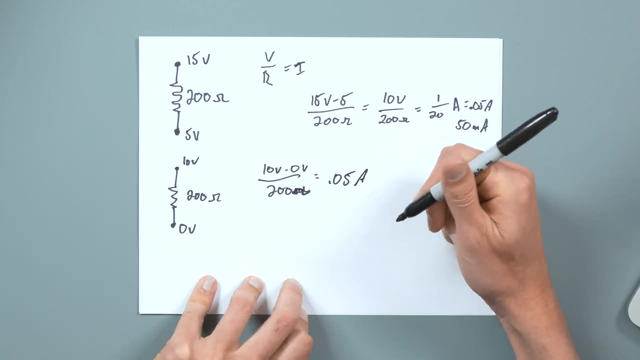 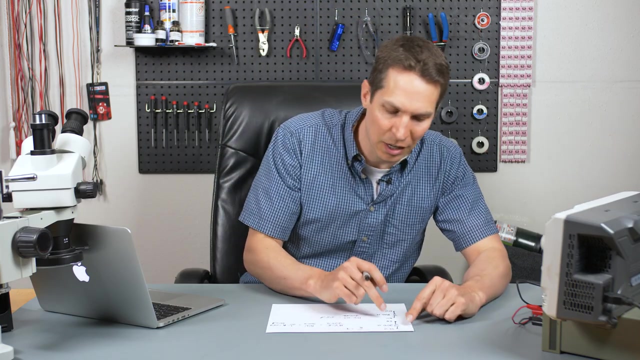 200.. Wow, That got out of control and that's still going to equal 0.05 amps. So that is what I wanted to do this for is just to show that voltage is all comparative. I could even go the other way around. 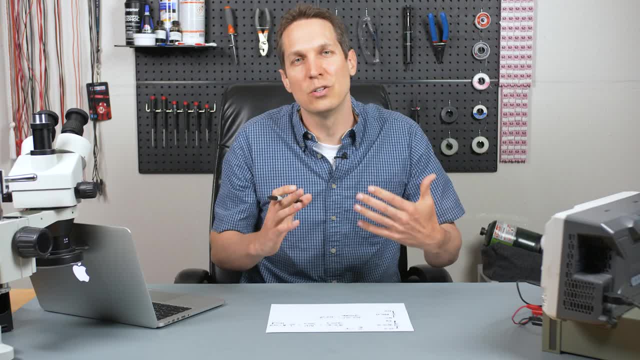 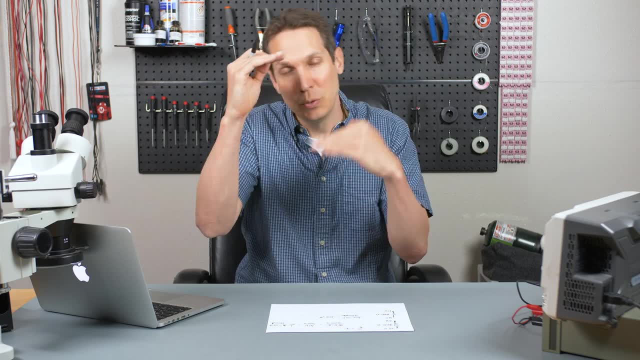 I could do that as negative 10 volts to negative 20 volts. It's still going to be the same thing. So voltage is all relative. It's that potential between or across between two points, across something else, So let's do another one. 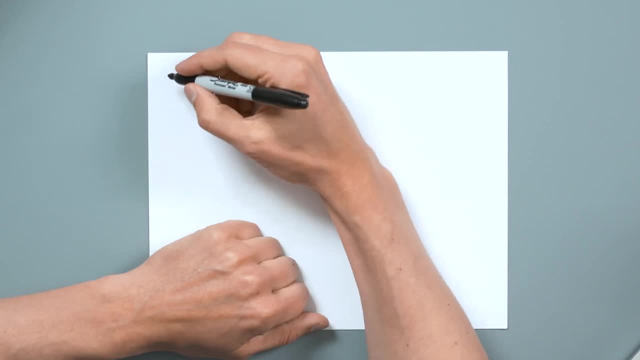 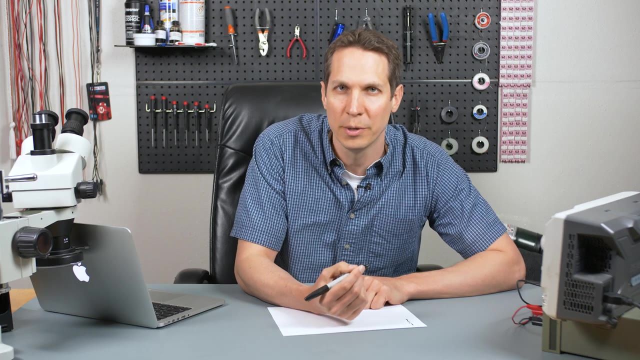 Okay, So two more quick examples. So this first one I am, and notice how I'm keeping these simple. I'm trying to keep the math simple because to me it's more about the intuitive understanding. You can use a calculator to get to do the crazy math, but if you want to be able to 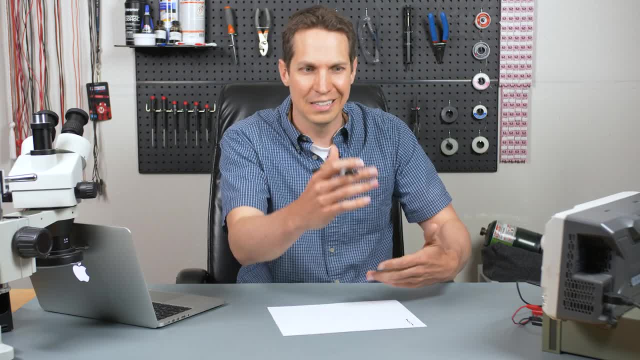 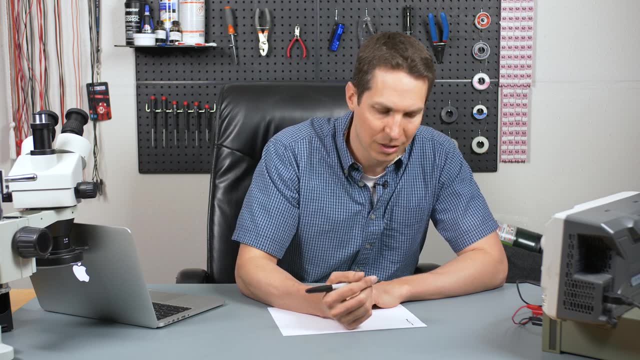 look at it and figure out how to solve it. you need to understand: Oh Hey, that's actually that way, I can flip that or I can move that and it won't actually affect anything. So that's, that's where I'm going with this. 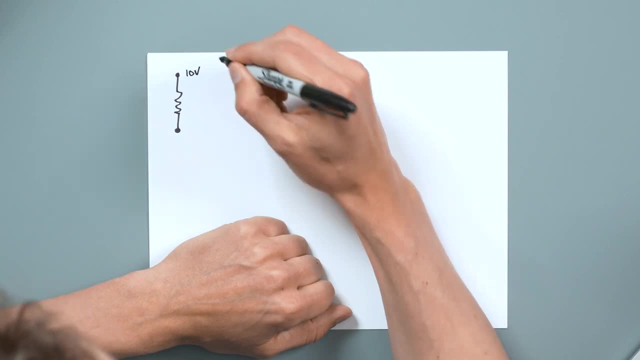 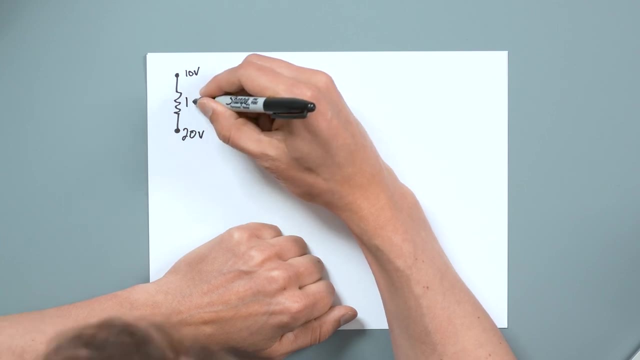 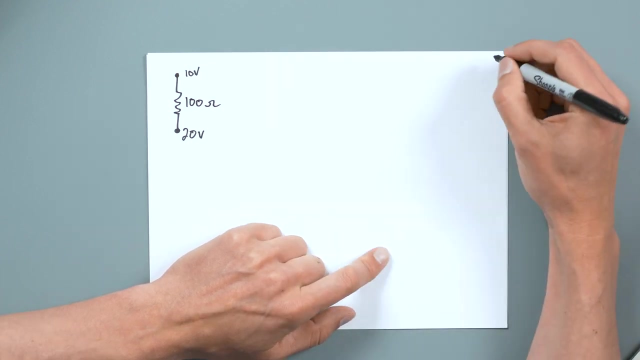 So let's actually assign this 10 volts and assign this 20 volts, and then we will say this is 100 Ohms, again, just for the fun of it. Okay, So now I'm going to set the equation up, and this is something I always did in college. 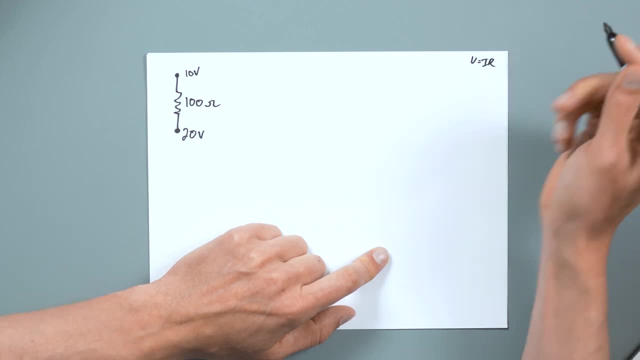 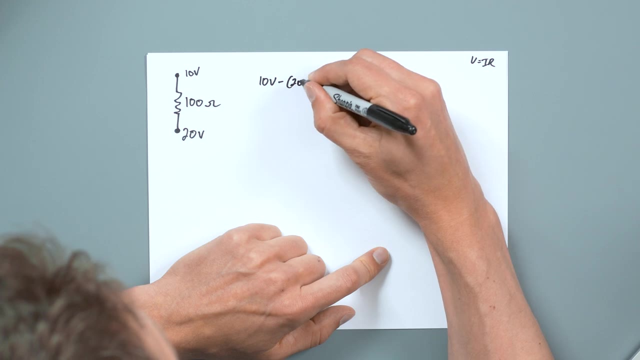 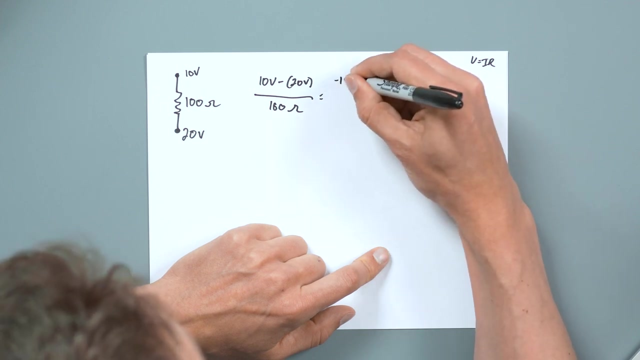 and I still do quite a bit. I'll just write Ohm's law in the corner, just to make sure that I'm not screwing anything up. So I'll have 10 volts minus 20 volts over 100 Ohms, which equals negative 10 volts over. 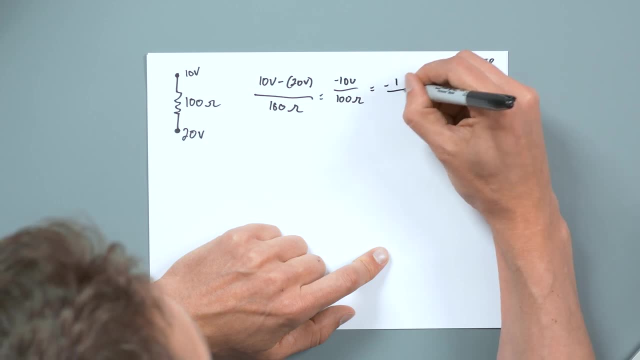 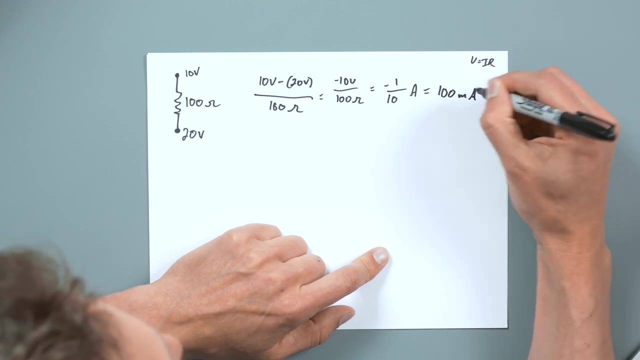 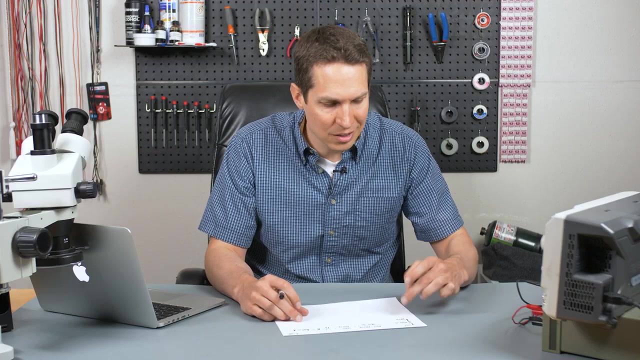 100 Ohms. What equals negative one? 10th, Okay, Amps or 100 milliamps. negative 100 milliamps, Okay. So negative 100 milliamps. What does that mean? Well, that means that we looked at this and the way it's set up, you'd imagine okay. 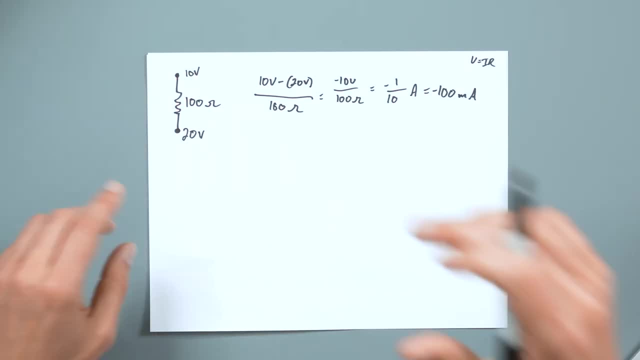 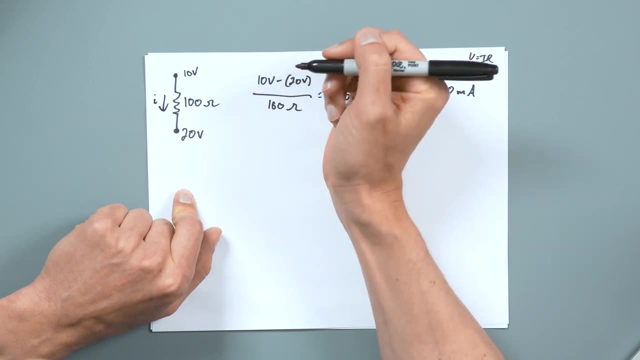 glass is up here, but actually this is completely flipped where the higher potential is down here. So, even though we have established that our current is going this way, in reality it's going the opposite way, But since we established that the current is going that way. 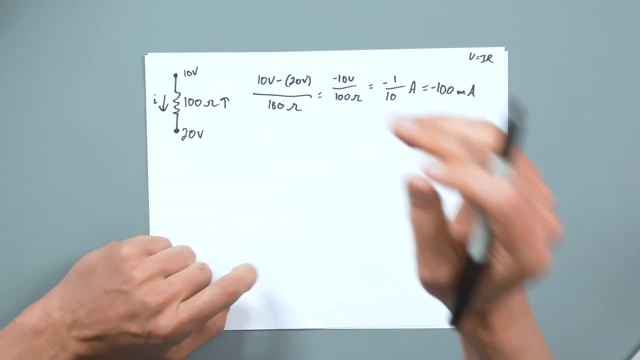 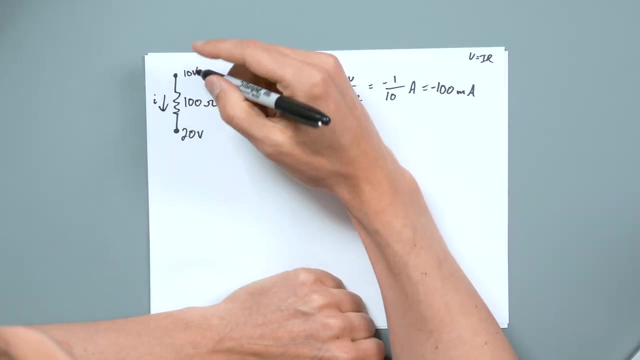 We want to say negative 100 milliamps, And that is an incredibly important thing to remember and something I still screw up with Ohm's law is you need to say. I am going to say that I'm going from this point to this. 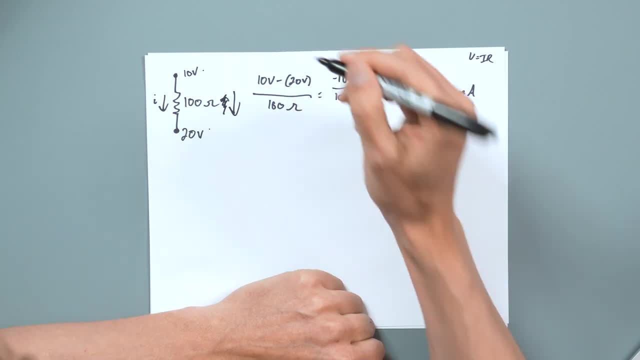 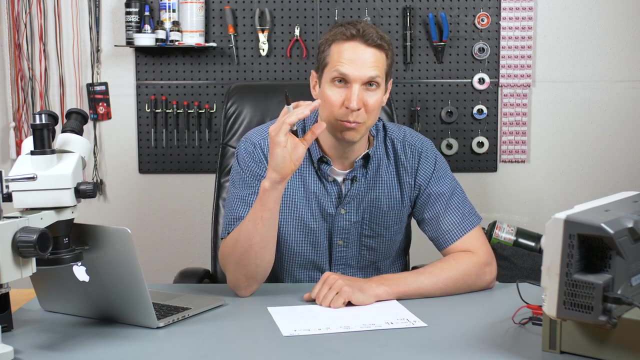 point. My current is going this direction and I am sticking with that. because if you say, Oh, that's negative, Well, let me just flip things around. You highly, highly increase the chance of you messing up your math somewhere. So what you do is you set up the equation, you look at it, you say, Hey, this is the 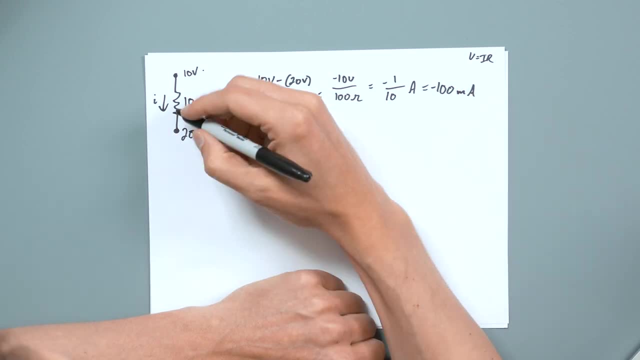 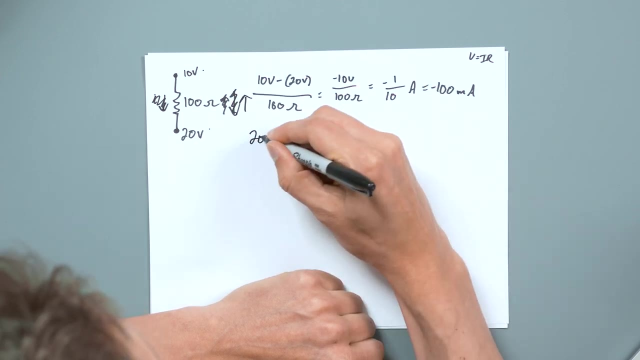 way it's going to be, And then I'm just going to take the signs as I go, Because if I take this and I switched it and I did all the math differently and went back up, then it would be okay: 20 volts minus 10 volts over 100 ohms. 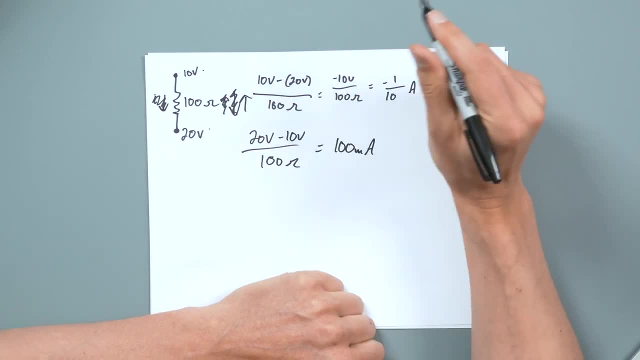 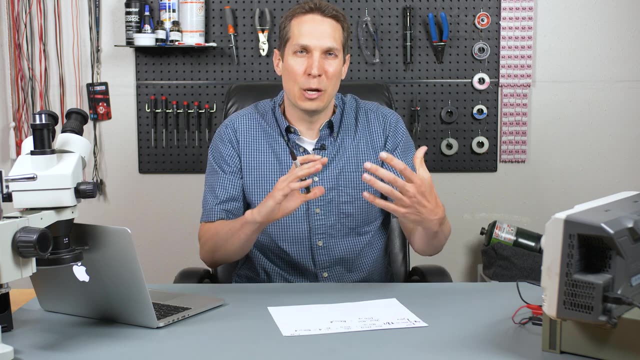 And then I'm going to get 100 milliamps, but it's going to be in the opposite direction. So that was the key with this one. that I want you to take away is that that positive and negative is a matter of perspective. 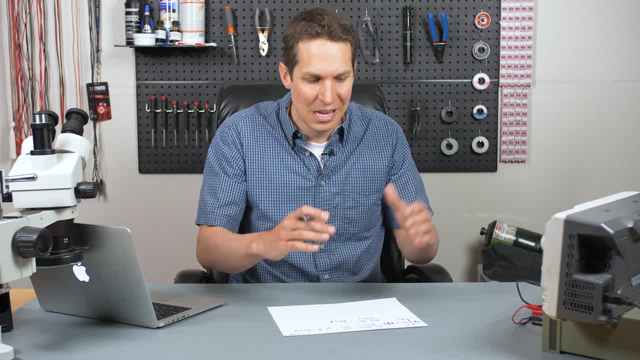 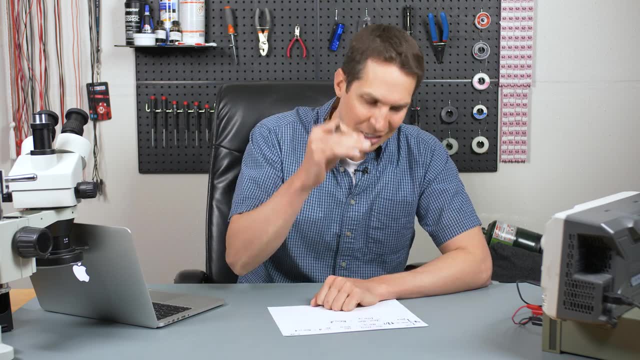 It's a matter of which way you're looking at it, So always keep that in mind And make sure that once you say I'm going to do this, I highly recommend writing it down on the paper as you're doing it. Once you say this is how I'm doing it, stick with it. 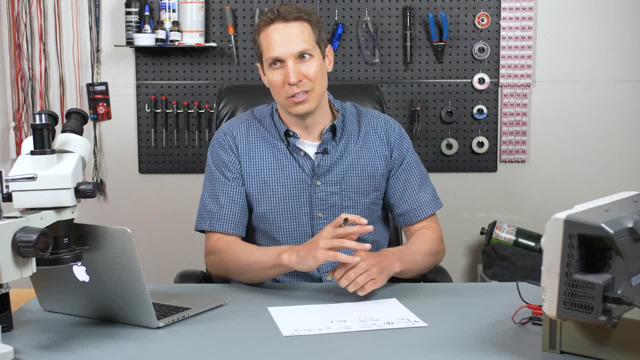 Don't switch it, don't change your mind, or else you're just going to confuse yourself. Or if you do switch your mind, switch your setup because you realize, oh man, that's going to be a complete nightmare. Just be very, very careful with that. 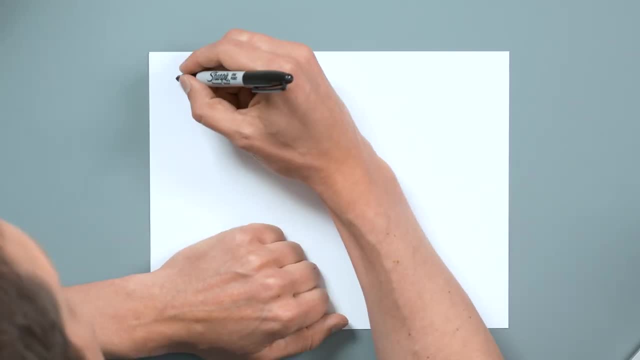 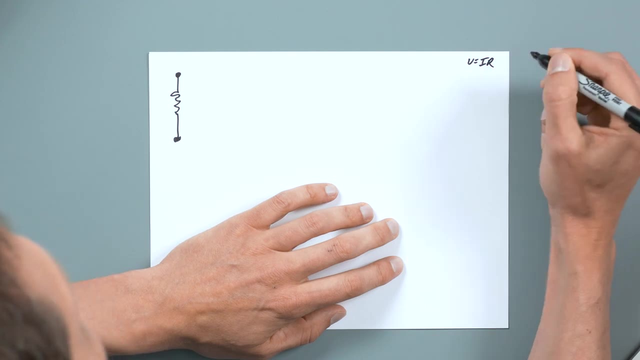 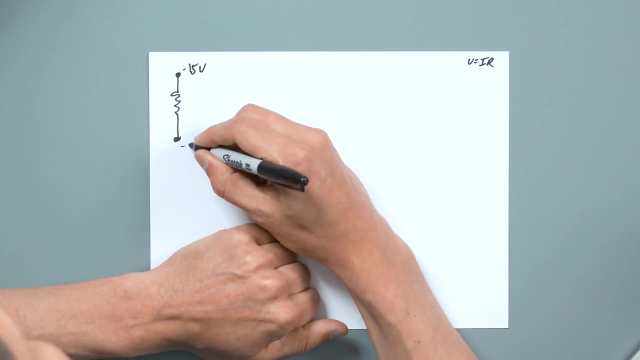 Okay, let's do one more. Alright, so this will be our last example. So let's do the same things we've been doing: the ugly resistor, the Ohm's law in the corner, and then let's just say: this is negative 15 volts and this is negative 25 volts. 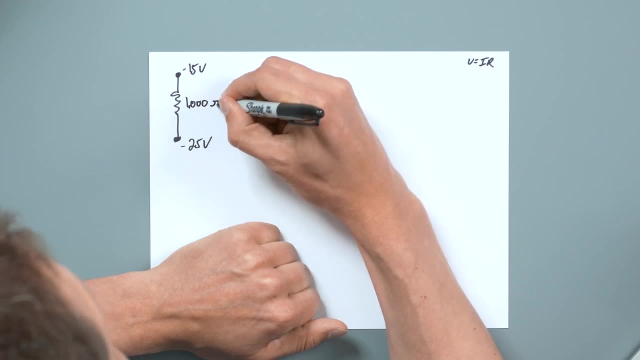 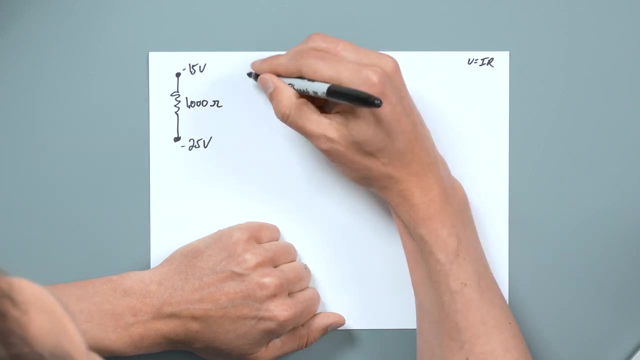 And then let's make this 1000 ohms, just because I'm getting bored with 100.. Okay, so we set up Ohm's law and we look at this and we say, okay, what's the difference between those? 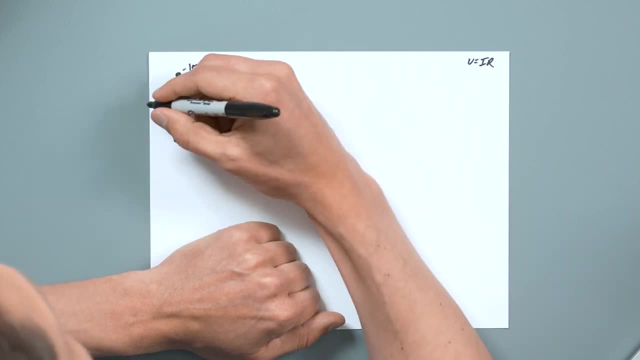 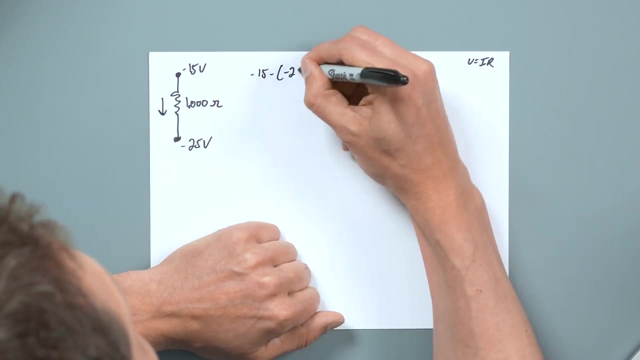 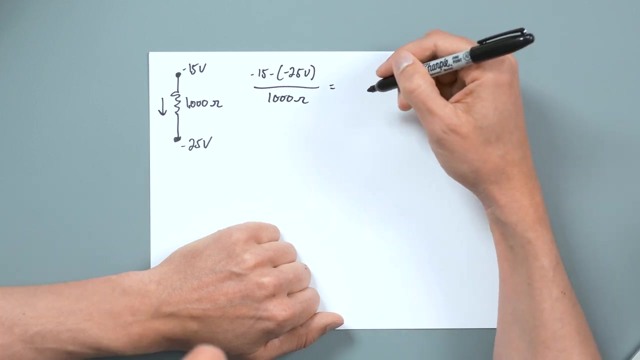 That's negative 15 volts. again, based off of what we just discussed, I'm assuming that our current is flowing down. So we've got negative 15 volts and then we've got a minus that one. So negative 15, minus negative 25 volts, and then over 1000 ohms. well, negative 15 minus. 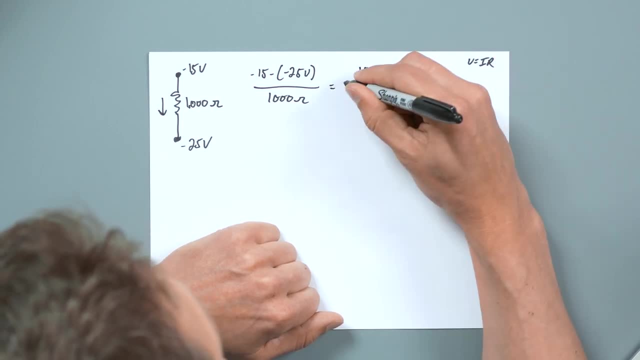 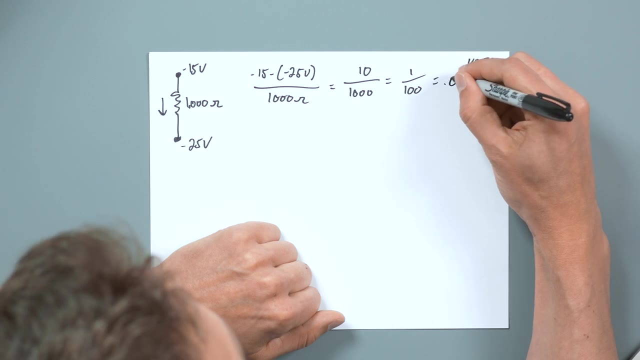 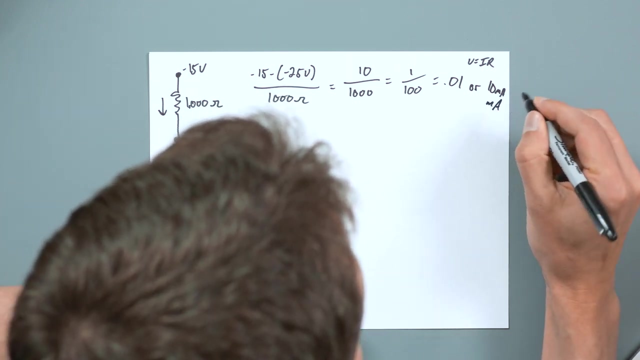 negative 25 is a positive 10. So that actually becomes a positive number. you got 10 over 1000,, which equals one over 100, which gives us point zero, one or 10 milliamps. Okay, maybe I should. just I'm gonna learn some great things while doing this about calm. 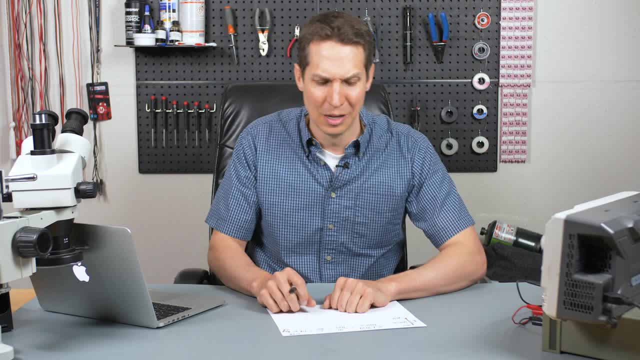 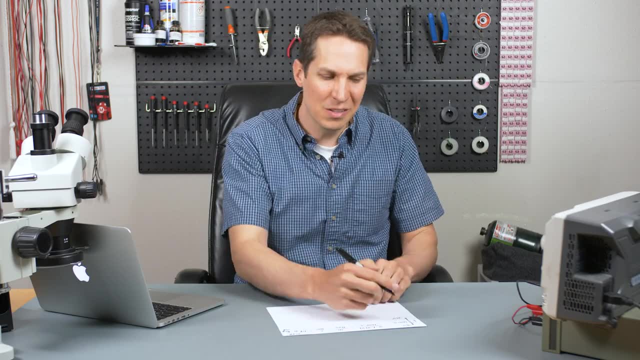 handwriting. Maybe everything will make sense, But the point I wanted to bring with this was again that different potential. it doesn't matter. So, even though this is a negative number and this is a negative number, it's all about the relationship between the two. 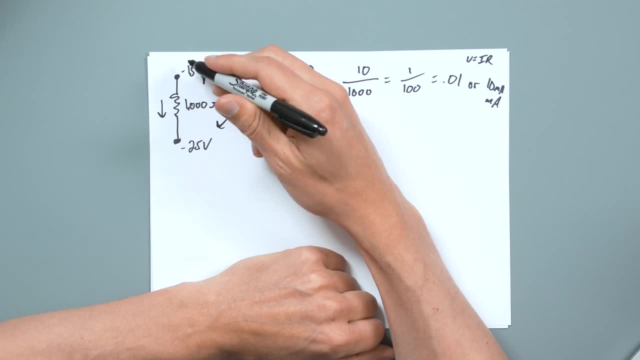 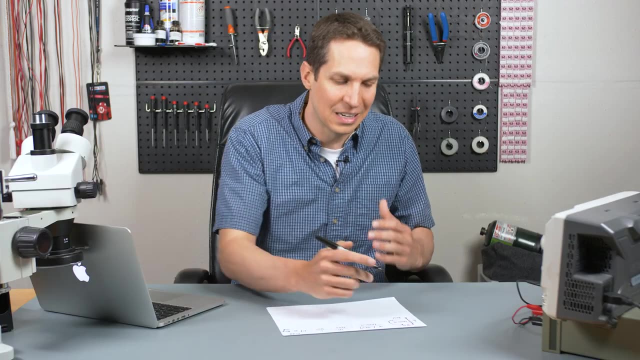 It's all about that voltage across this. So just because this is negative 15 and negative 25, in this case because there's nothing else- those numbers are basically arbitrary. Again, you could go and have 10. And zero, and it acts the exact same way.